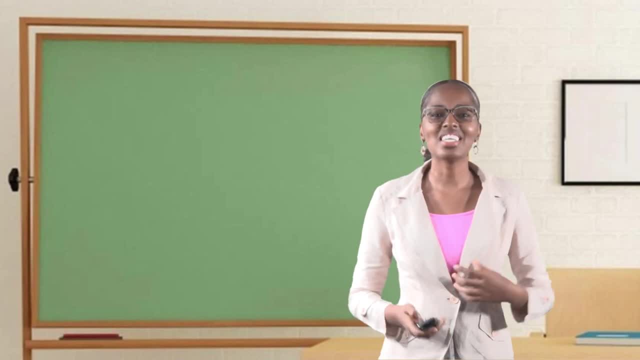 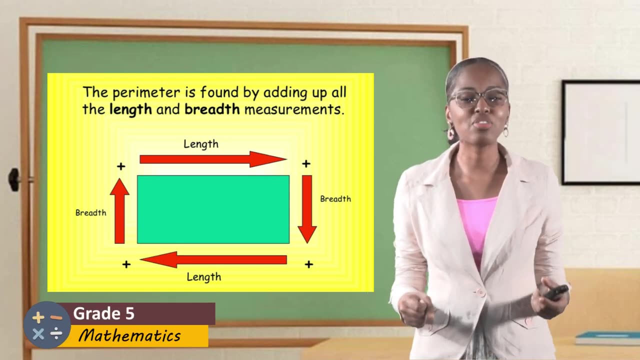 I hope you enjoyed that song, boys and girls. Now let's move on to recap what perimeter is. Okay, boys and girls, from that song you would have noticed that perimeter is about adding all the sides And really and truly, perimeter is the measurement. 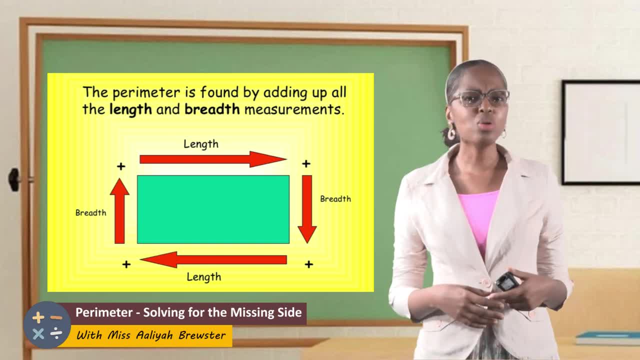 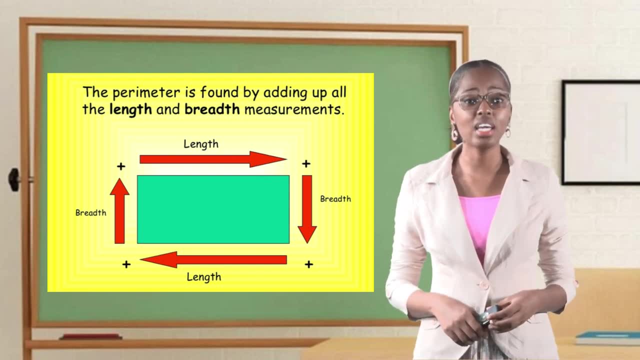 or the distance around a plane shape. How do we calculate perimeter? Perimeter can be found, of course, by adding all the sides, or some persons like to say by adding the length and the breadth of the shape. For example, if you have a rectangle, 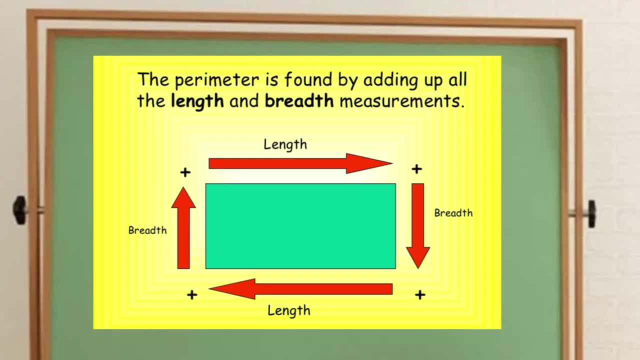 remember, a rectangle has two long sides, two parallel lines then that run horizontally, or two long sides, and then they have two short sides, which would be two vertical parallel lines. To find the perimeter of a rectangle, we add all four sides To find: 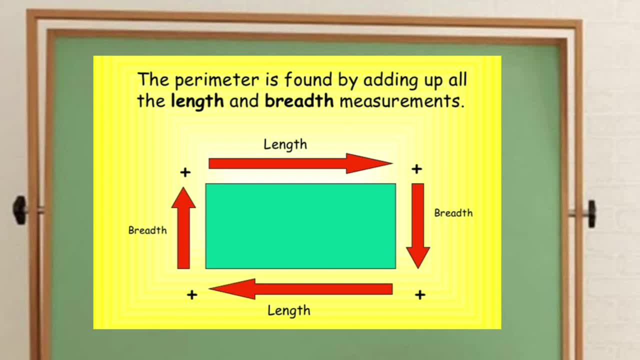 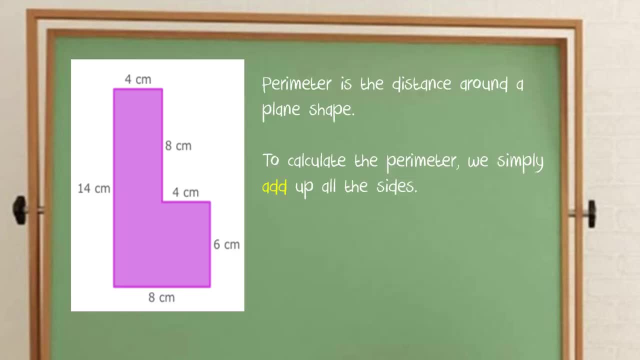 a perimeter of any shape. we simply have to add all the sides together. Let's practice In this case. we're given a shape that looks like the letter L and we're tasked to calculate the distance around that shape. To calculate the distance, we of course add all the sides. 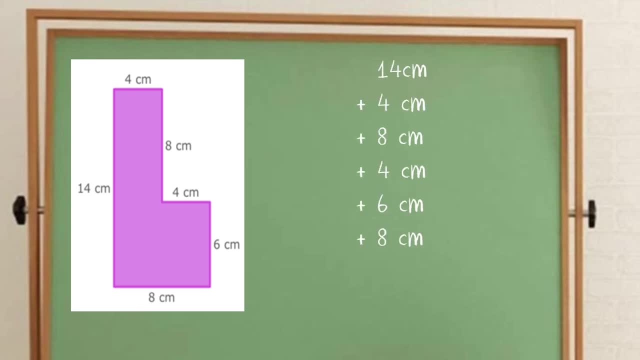 In this case we add 14 centimeter, 4 centimeter, 8 centimeter and 10 centimeter, 8 centimeter, 4 centimeter, 6 centimeter and 8 centimeter again, and that would give us 4 to 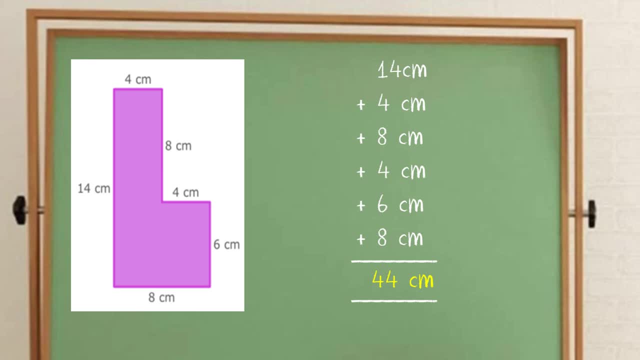 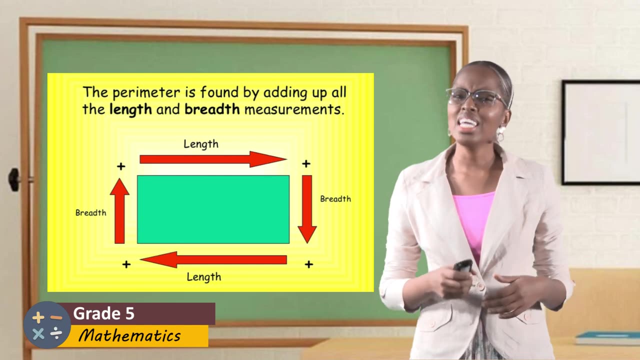 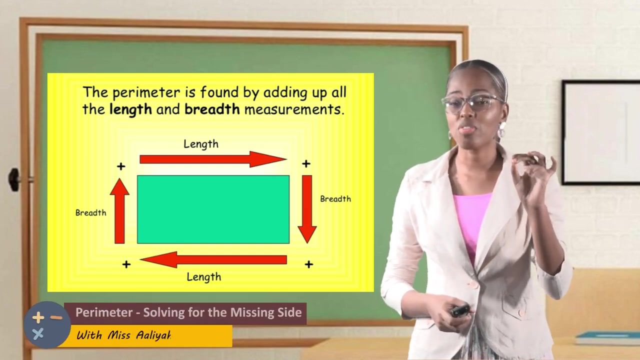 4 centimeter. Therefore, the perimeter for that shape would be 4 to 4 centimeter. That's what you learned, because I taught you that. However, there are instances where perhaps we're not really given the entire measurement of the shape and we have to do some critical thinking. For example, 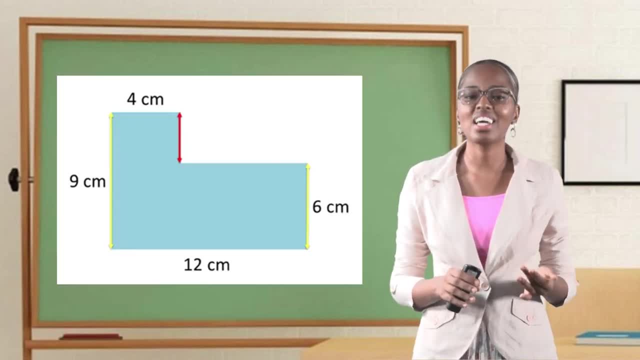 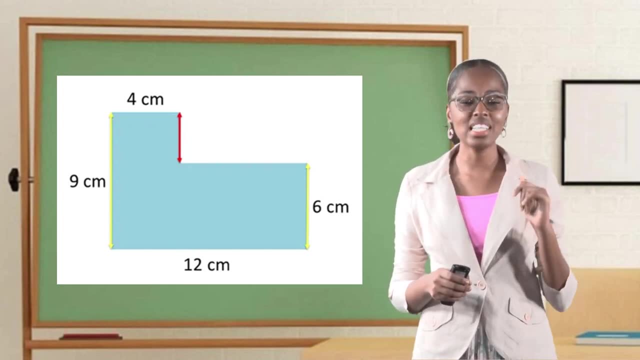 if you look closely there's another shape. It looks like a L again, but a funny-looking shaped L, And at the corner we have 9 centimeter. At the top we have 4 centimeter and at the bottom 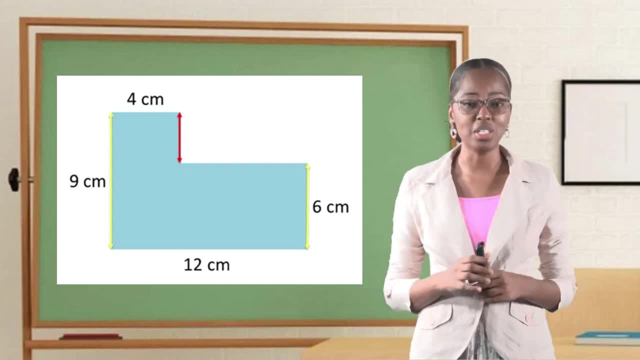 we have 12,, while at the other side we have 6 centimeter. Now, if I were to ask you to calculate the perimeter for that shape, you would, of course, add 4,, 9,, 12, and 6.. 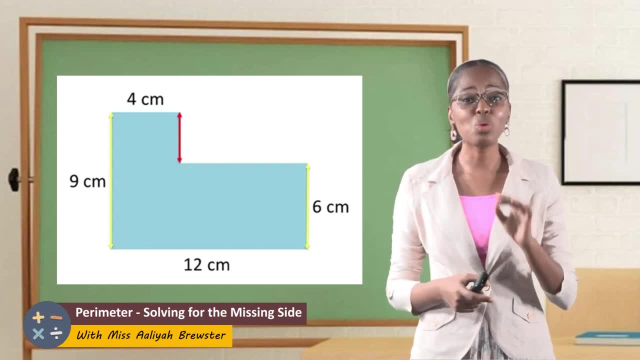 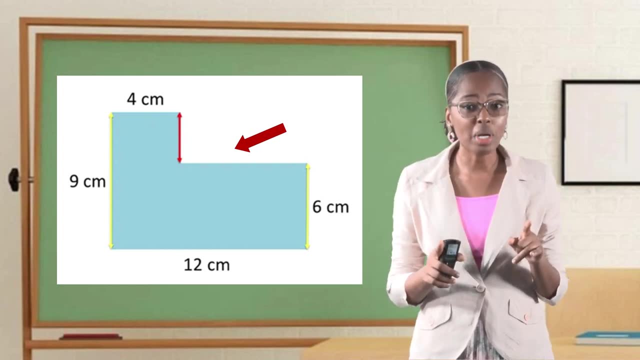 But wait a minute, There are some parts missing. We don't know the measurement for the part of the shape that has a red line on it, nor do we know the measurement for the part that goes across. That's just above the 12 centimeter. Therefore, we have to do a bit more calculating, It's not? 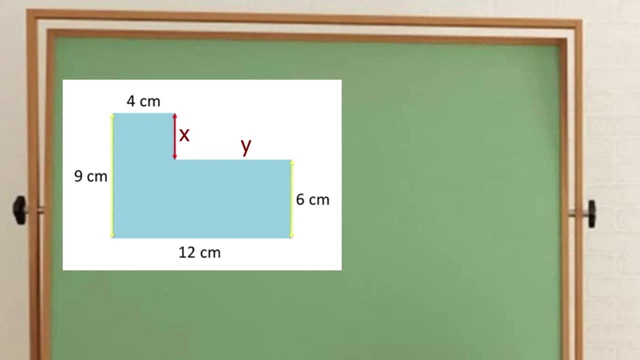 difficult. I'm going to show you an easy way. Okay, So to solve for the missing sides, we label them. One side we label it X and the other side we label it Y. If we're going to solve for X, we have to look at the shape. 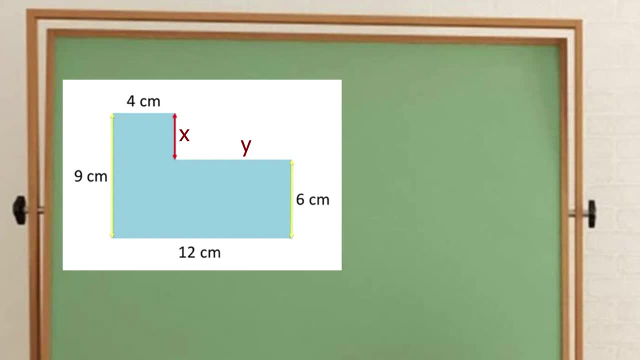 in its entirety And if you notice that shape, it resembles a rectangle, meaning that the sides, the lines that are at the top and at the bottom, are parallel horizontal lines and they should be measured the same, while the lines that are at the two sides are. 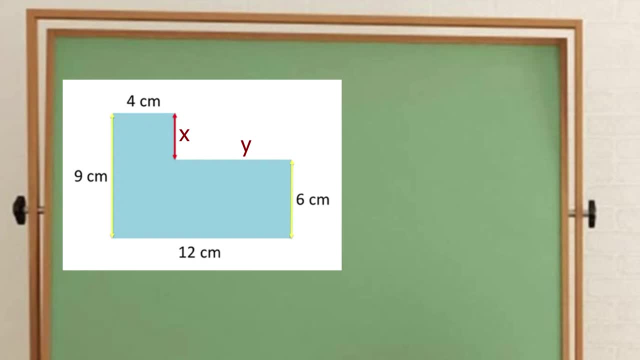 vertical parallel lines, and they too are measured the same. However, the lines that are this way and this way doesn't necessarily need to have the same measurement. That's a square, Remember. a square has equal sides. All the sides are measured the same. But a rectangle, the two longer sides have. 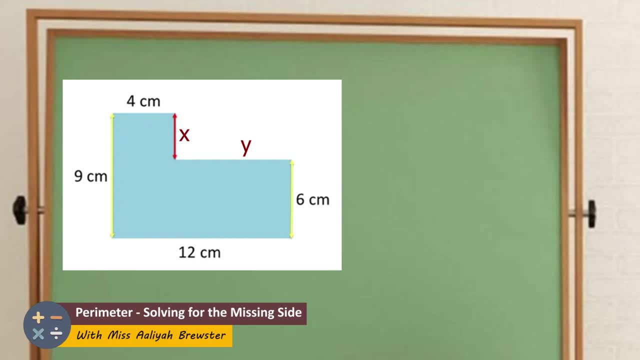 one measurement and the two shorter sides have another measurement. Bearing that in mind, look at the shape again closely. To solve for X, we must look at the two parallel lines that are vertical or they're pointing upwards, And that would be the ninth centimeter and the 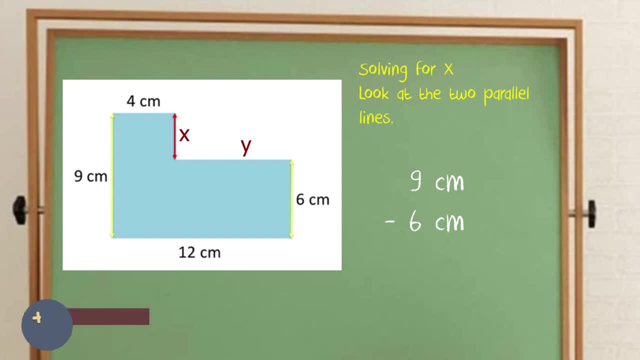 sixth centimeter. So if we're going to solve for X, we have to minus six centimeters from nine centimeters, Because you remember a rectangle- the two lines at the side are equal. They're equal. Therefore, we can assume that if one side- the entire side- is nine centimeters, then the other 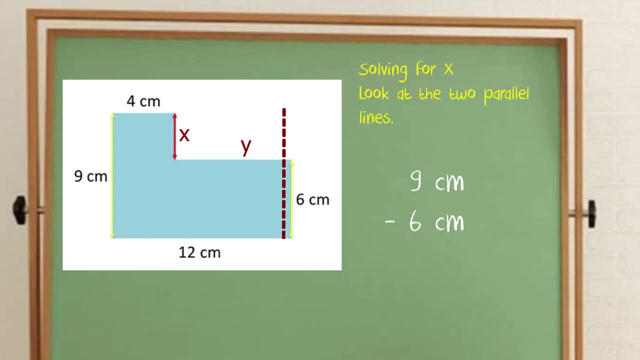 side should measure up to nine centimeters as well, And that would be inclusive of the six centimeters as well as the other side. Now, even when we're going to solve for X, we have to look at the shape of the rectangle in its entirety, meaning that the sides are equal. They're equal. Therefore. 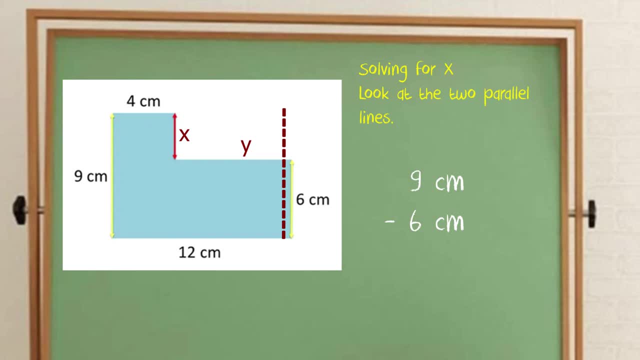 as the value for x. So when we add x and 6 cm we should get 9 cm, But because we don't know the value for x, we have to minus. So we minus 6 cm from 9 cm and that would give. 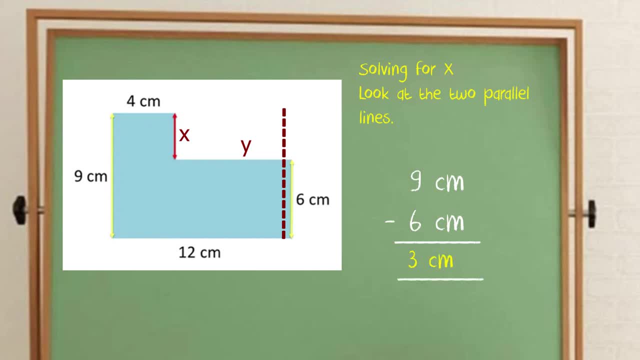 us the value for x, And the value for x, therefore, would be 3 cm, And that's because of the vertical parallel lines. Good, If we're going to solve for y now, or to find the exact measurement for y, we look at the lines that are going in this direction. They're horizontal. The. 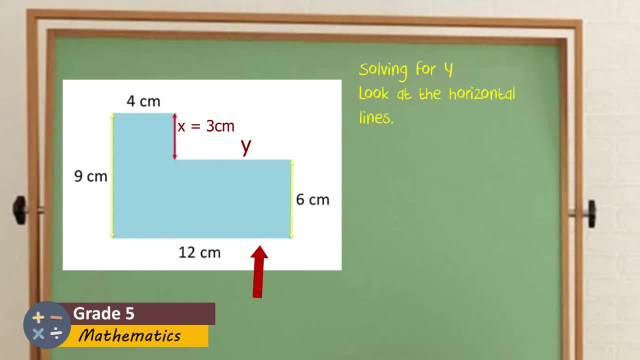 perpendicular lines that are going like this Right. So the bottom line there is measured at 12 cm. Therefore, the measurement for the top should be 12 cm as well. However, because of how this shape is situated, 4 cm has to be subtracted from the bottom line, So we 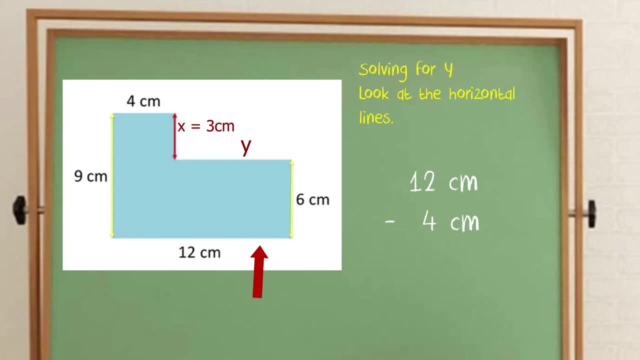 minus 4 cm from 12 cm to give us the value for y, Because 4 cm plus the measurement of y should be equivalent to 12 cm, Because, remember a rectangle- the two sides at the top should be the same. Okay, We minus 4 cm from 12 cm and that will give us 8 cm. Therefore, it 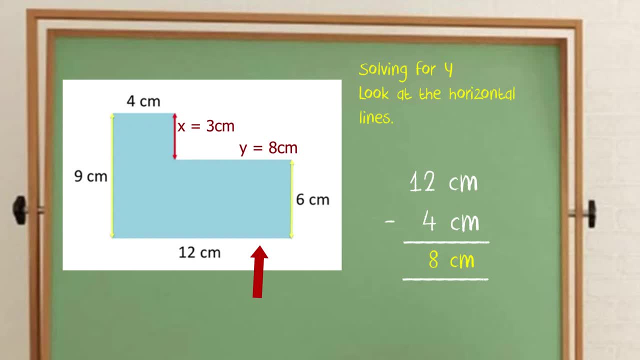 is safe for us now to calculate the perimeter for the entire shape, Because we know that what's the measurement for x and y. So we add 9 cm, 4 cm, 6 cm, 12 cm and 3 cm which. 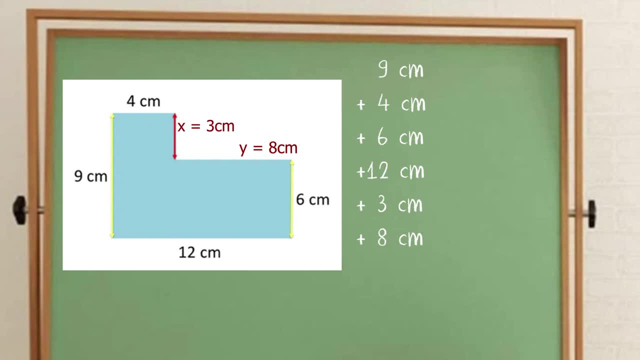 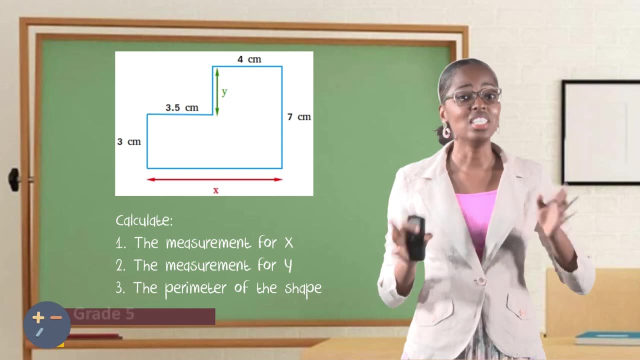 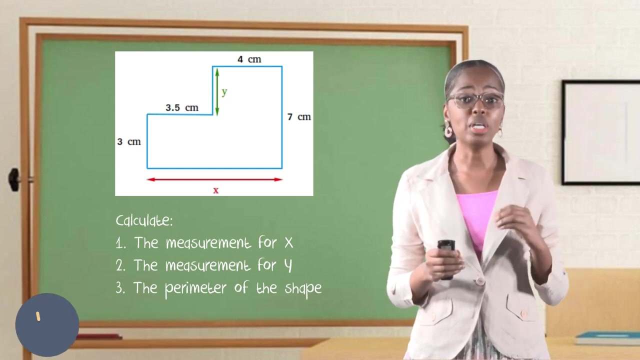 is the value for x, and 8 cm, which is the value for y, And that would give us 42 cm. Let's try another activity. This time I'm going to allow you to do this on your own, and then I'll explain. For this task, you're going to calculate the measurement for x. 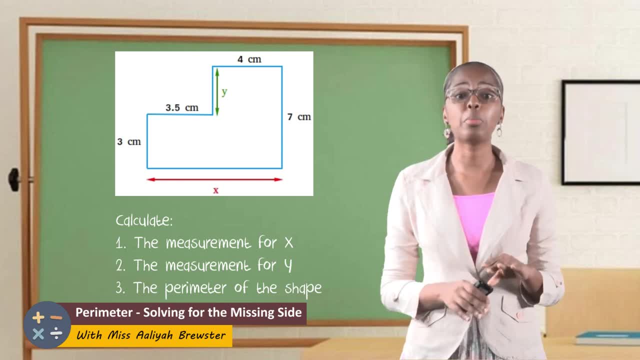 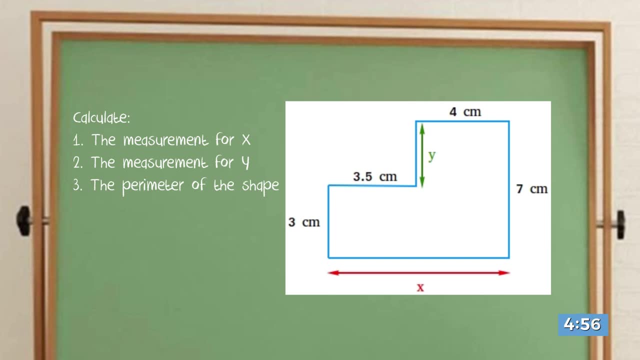 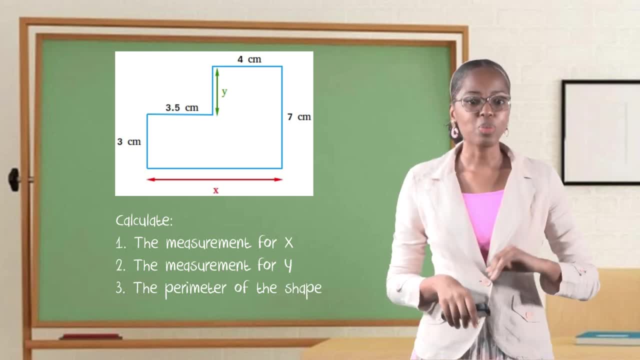 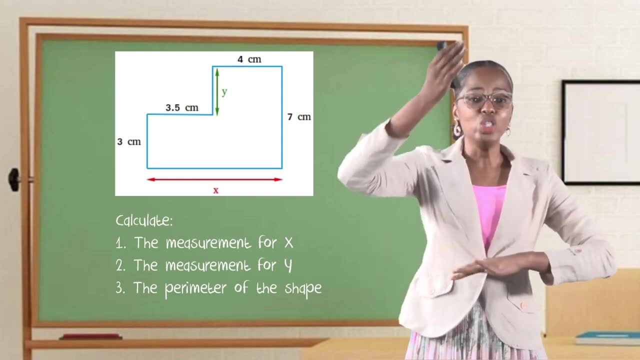 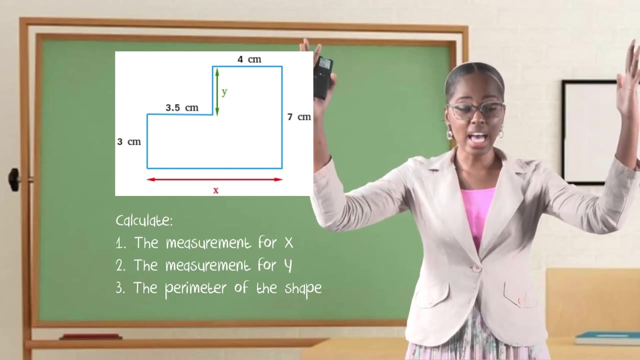 Let's verify. To solve for X, we look at the shape And again this shape resembles a rectangle, meaning that the two lines at the top should be equal to the same measurement, and while the lines at the two sides should be equal to the same as well. 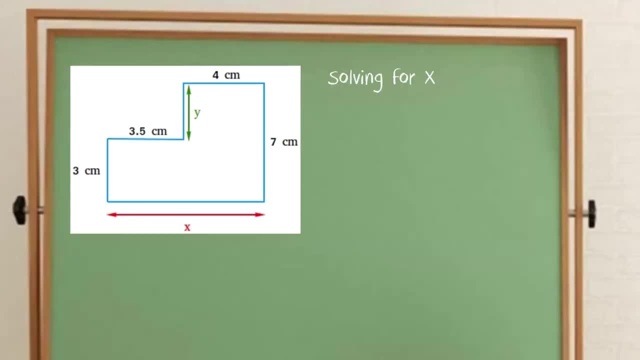 So if we're going to solve for X, we look at the top of the shape there And if you notice, at the top there's one measurement going up this way which is 4 cm, and then there's another one just below that which is 3.5 cm. 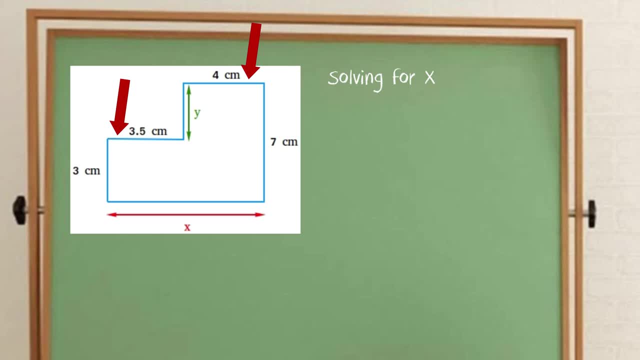 However, let's say both of those lines were on the same level, the 4 cm and the 3 cm. That would give us the measurement for X. So what do we do? We add 4 and we add 3.5.. 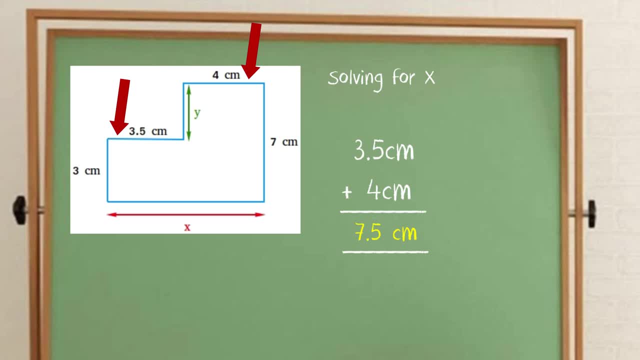 And when we do that, we get 7.5.. Therefore, the value for X would be 7.5 cm. Now let's solve for Y. To do this, we look at the lines that are at the side and that are running vertically. 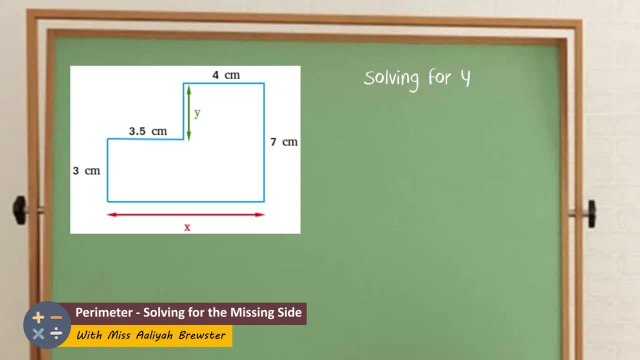 We have 7 cm and 3 cm. Of course this side is equivalent to this side. So if we were to find for Y, we have to minus 3 cm for 7 cm And that would be 4 cm. Therefore the value of Y or the measurement of Y is 4 cm. 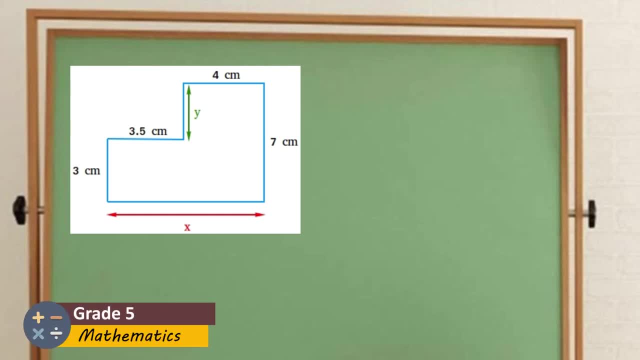 Now it's safe for us to calculate the perimeter of the entire shape because we have all the measurement for every side of this shape. So we add 3 cm plus 3.5 cm plus 4 cm plus 7 cm And the value for X, which is 7.5 cm. 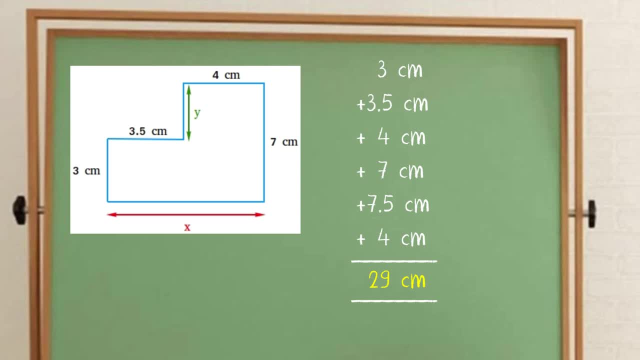 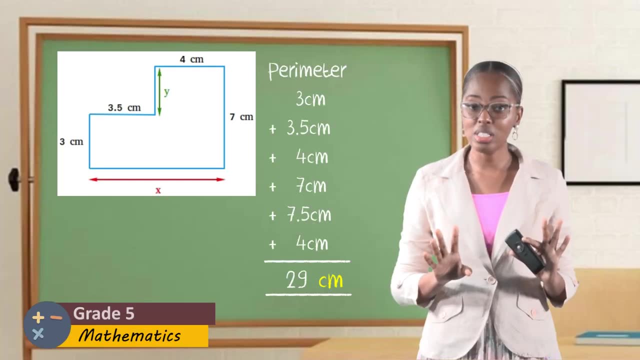 and we add the value for Y as well, which is 4 cm, And that would give us 29 cm. If you notice closely in the answer, I didn't just write 29 and leave it that way. You have to write the unit of measurement that you're using. 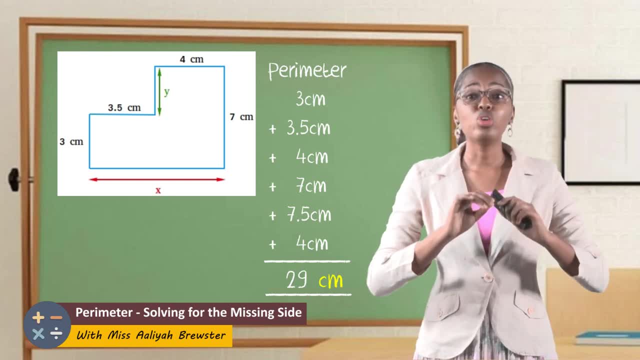 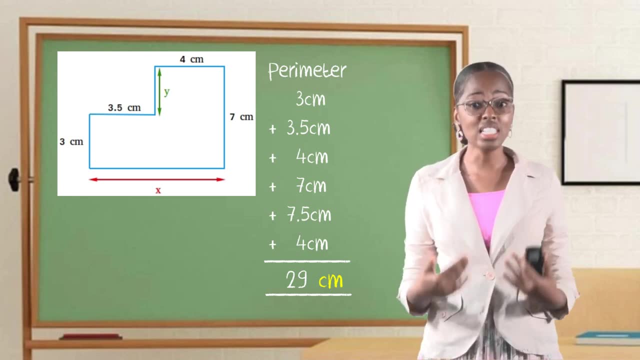 Whether it is cm, m, whether you're using inches or feet, whatever it may be, in your answer, you have to write back that unit of measurement. In this case, our unit of measurement is cm, So the answer would be 29 cm.